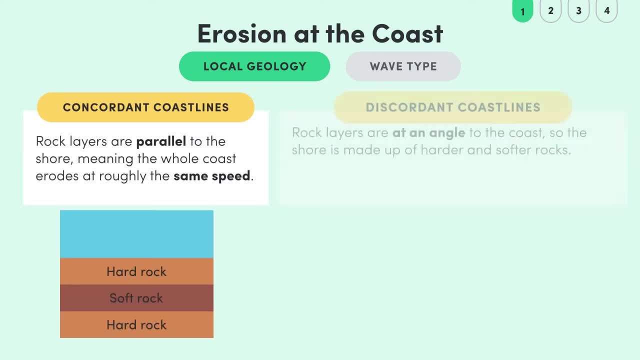 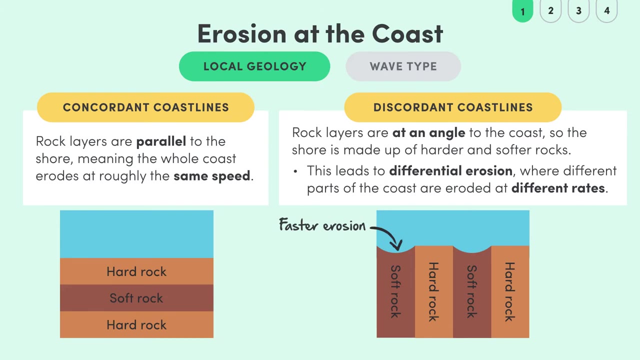 A discordant coastline is one where the rock layers are at an angle to the coast, so the shore is made up of harder and softer rocks. This leads to differential erosion, where different parts of the coast are eroded at different rates. Another factor is the type of waves found at the coast. 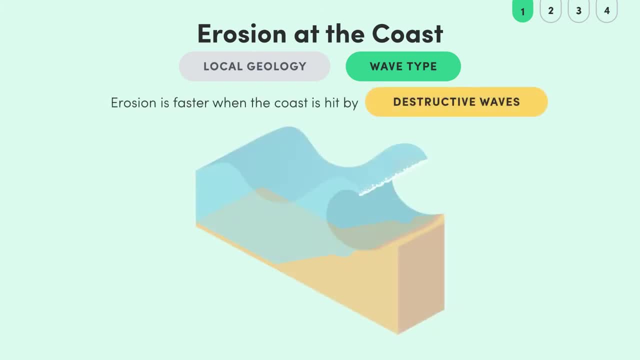 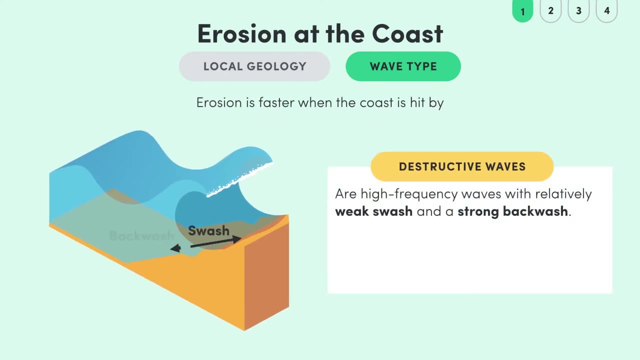 Erosion will be faster if the coast is hit by destructive waves. These are high frequency waves with a relatively weak swash and a strong backwash. What this means is that these waves hit the coast quickly and can pull lots of sediment away with them. 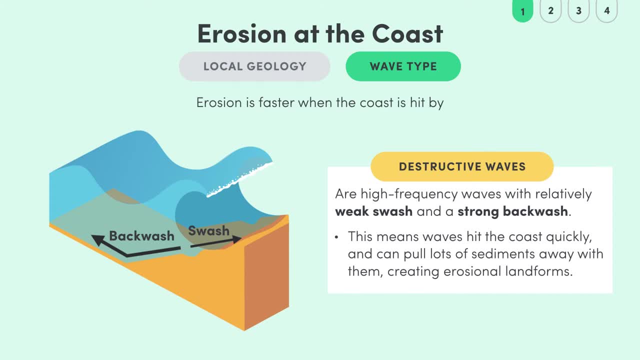 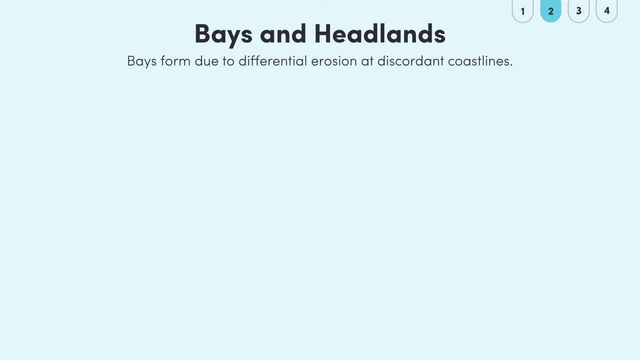 creating landforms of erosion rather than landforms of deposition. So how do these factors affect which landforms are created? Let's take a look at our first landform: bays. Basically, bays are the result of differential erosion at discordant coastlines. 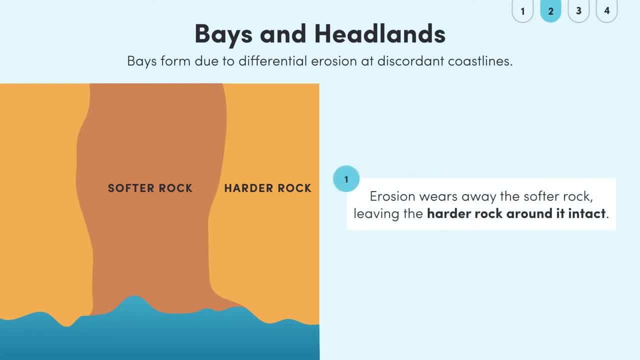 Erosion wears away a lot of sediment. This is due to the fact that the rock layers are at an angle to the coast, so the coast is more likely to be eroded at different rates. This is due to the fact that the rock layers are at an angle to the coast. 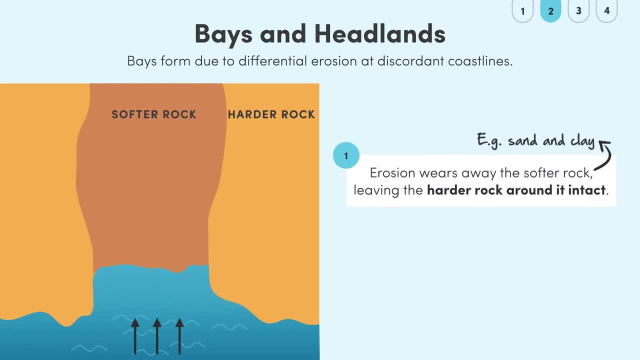 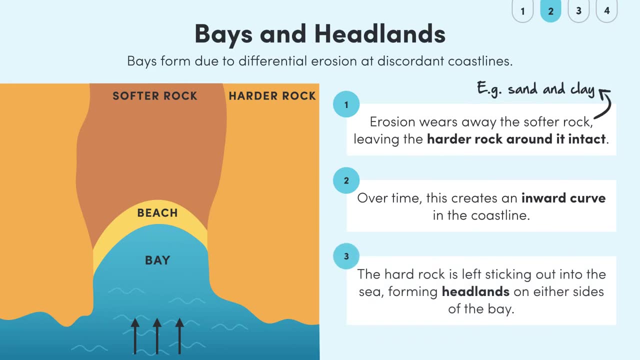 so the coast is more likely to be eroded at different rates Over time. this creates an inward curve in the coastline – a bay. The hard rock is left sticking out into the sea, which forms headlands on either side of the bay. 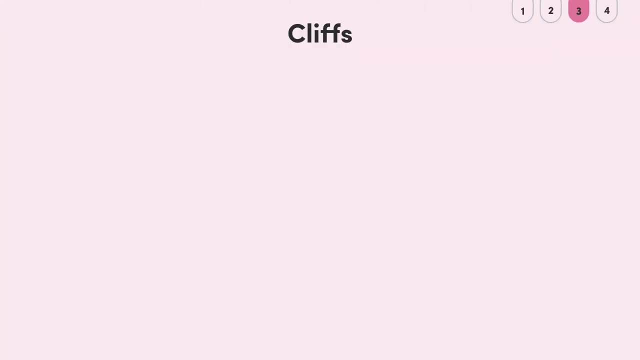 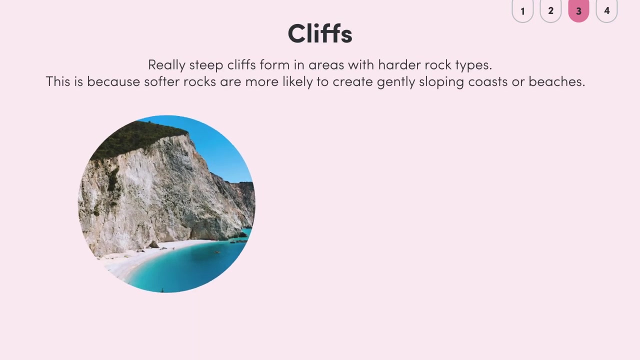 Cliffs are another common coastal landform. Really steep cliffs only tend to form in areas with harder rock types. Soft rocks are more likely to create gently sloping coasts or beaches. A great example of this are the White Cliffs of Dover – extremely steep cliffs. 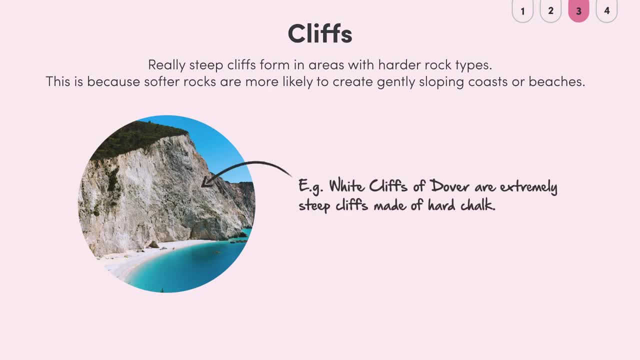 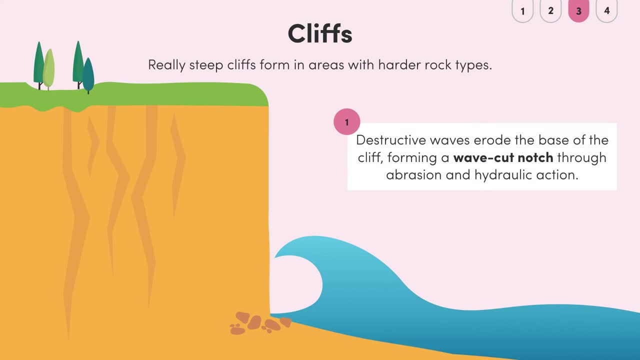 which are made of hard chalks. Cliffs have a particular pattern of erosion that you'll need to learn. Destructive waves can only erode the base of the cliff, causing the formation of a wave cut notch through processes like abrasion and hydraulic action. 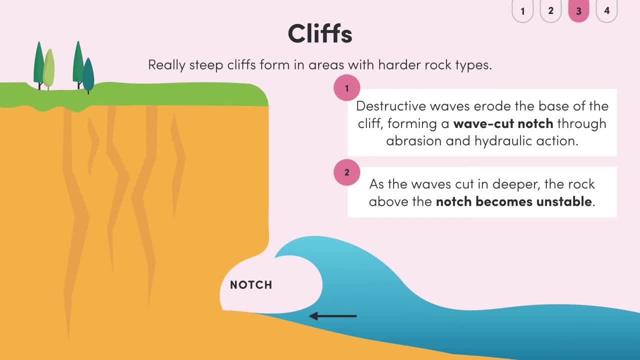 The deeper the waves cut into the cliff, the more unstable the rock above the notch becomes. Eventually it gets too heavy and unstable and the cliff collapses into the sea, forming a wave cut platform just under the waterline. Then the cycle begins again as a new wave cut notch begins to form. 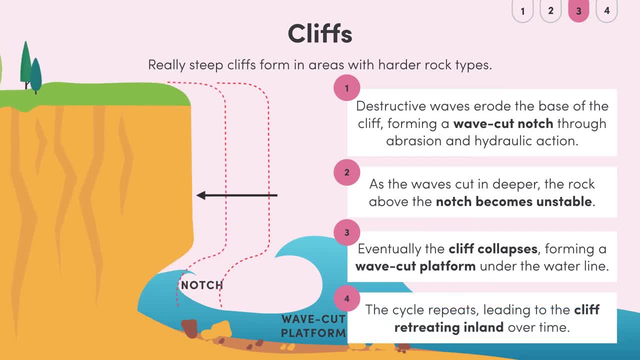 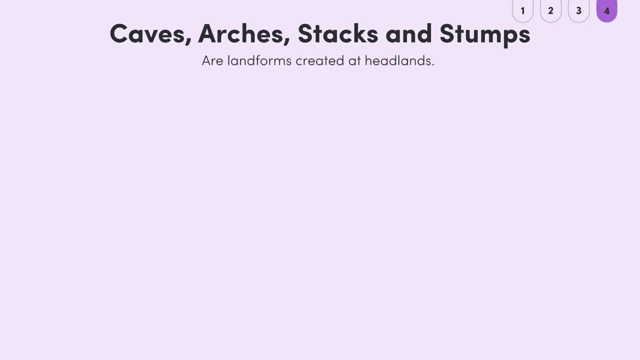 Over time, this leads to the cliff retreating inland. Another series of important landforms of erosion are created at headlands. These include caves, arches and ponds. These include caves, arches and ponds. These include caves, arches and ponds. 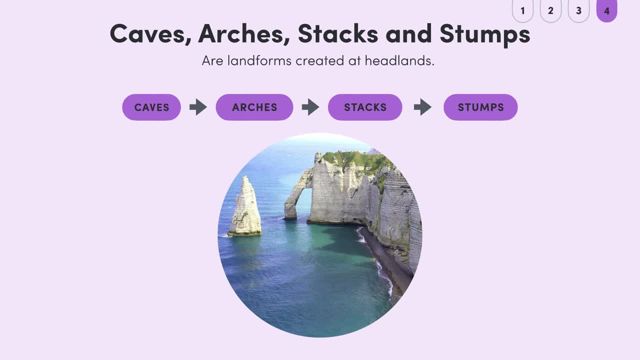 These include caves, arches, stacks and stumps. Headlands are particularly vulnerable to erosion by waves because they stick out into the sea. This means that cracks in the rock are hit with lots of abrasion and hydraulic action, making them larger. 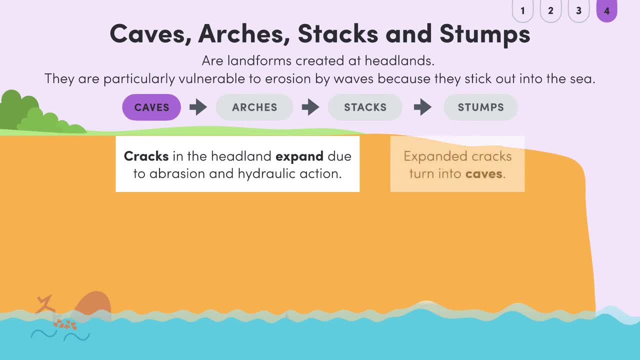 As those cracks become even larger, they eventually form into caves. These caves can then continue to extend through the headland until they eventually break through the rock at the other side. This creates an arch of rock. This creates an arch of rock. However, erosion still continues to wear away at the rock forming the arch. 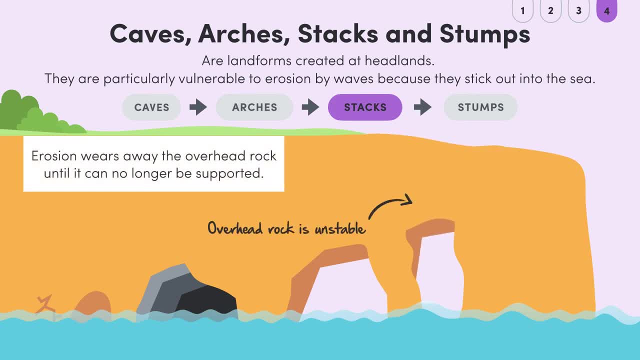 making it bigger until it can no longer support the rock at the top of the arch. This rock then collapses into the sea, leaving the headland on one side and an isolated column of rock known as a stack. Finally, even the stack is undercut by wave action in a similar manner to a cliff. 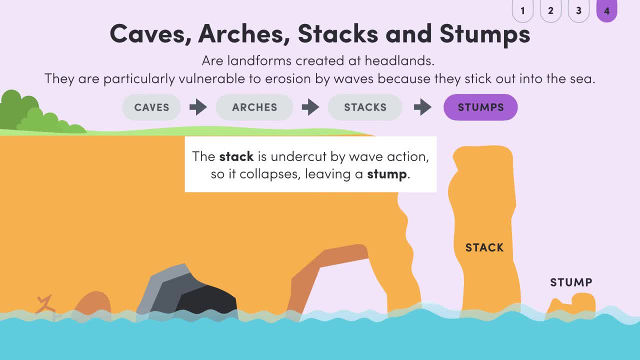 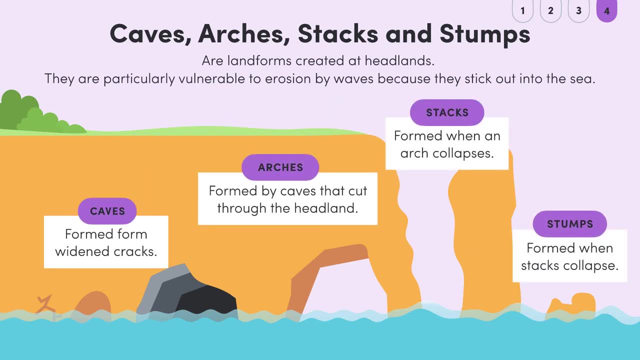 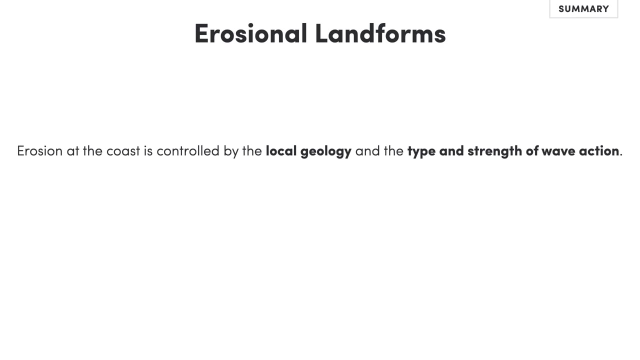 This weakens and collapses the structure, leaving only a stump of rock, And that's our lesson on erosional landforms at coasts. Let's go back over what we've learnt for your notes. Erosion at the coast is controlled by the local geology and the type and strength of wave action. 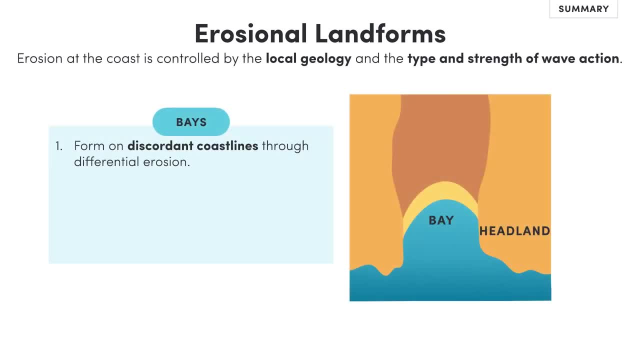 Bays form on discordant coastlines through differential erosion. Softer rocks are eroded more quickly than harder rocks, creating an inlet in the coastline and leaving harder rocks sticking out to sea. Cliffs are usually found in areas of harder rock. 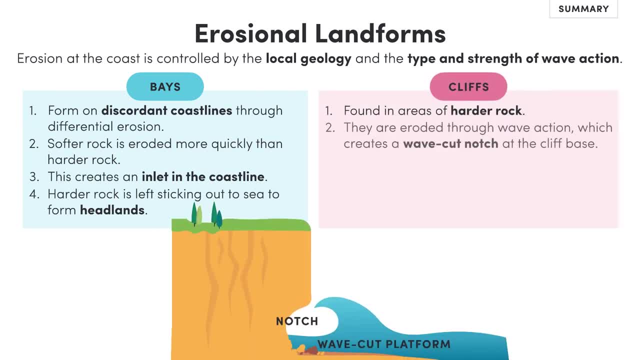 Cliffs are eroded through wave action, which creates a wave-cut notch at the base of the cliff. Eventually, the cliff collapses and the rock is washed away, creating a wave-cut platform and pushing the cliff further. inland Headlands have their own specific landforms. 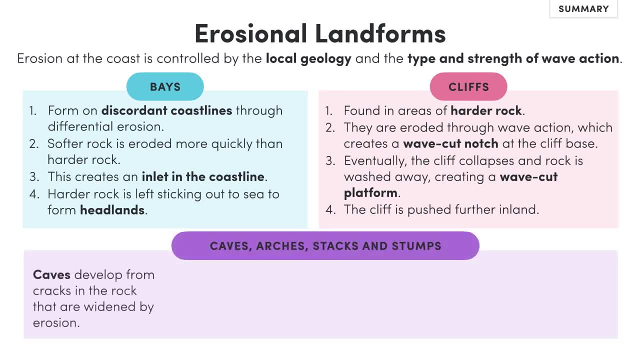 Caves develop from cracks in the rock widened by erosion. As the cave gets larger, the rocks are more likely to collapse. The rocks are more likely to collapse If the cave gets longer. it can cut straight through the headland to form an arch. 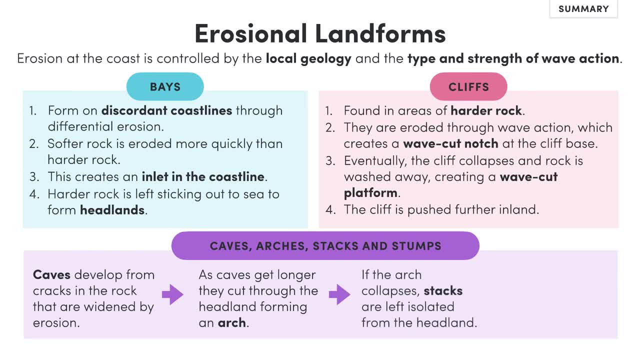 If the arch collapses, columns of rock are left isolated from the headland. We call these columns stacks. Finally, the stacks can collapse to create a stump, So that covers erosional landforms at coasts. Next up we'll cover coastal landforms formed by deposition.